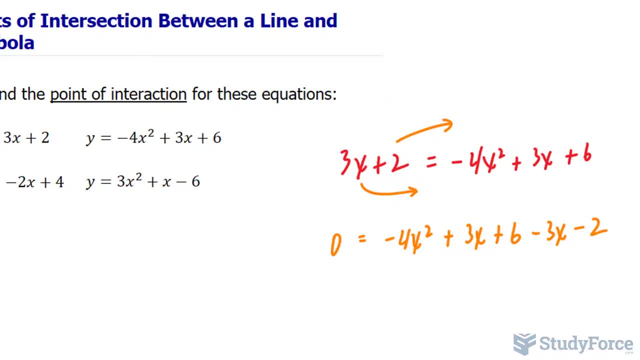 And the same, with positive 2 becoming negative 2.. We'll collect like terms and combine So this and that will come together: Positive 3x minus 3x makes 0.. Technically we got lucky here, Because sometimes, after combining the x terms, 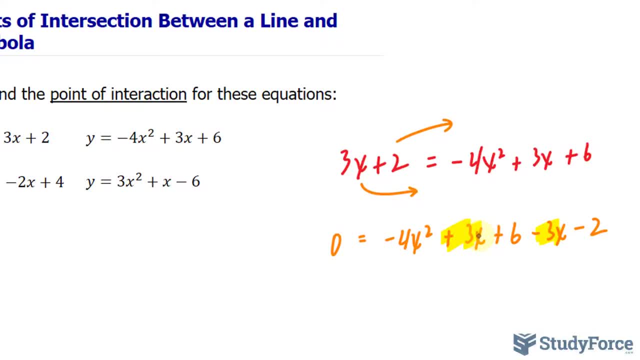 you don't get 0. But instead some other number. In that case, you would have to use the quadratic formula to find the x values following this step. In fact, you'll see that in example b, So I'll just cancel them out. 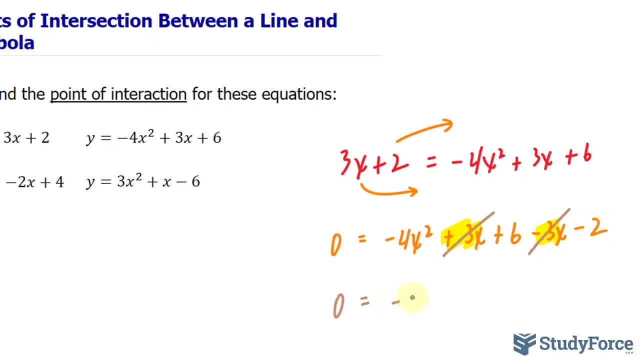 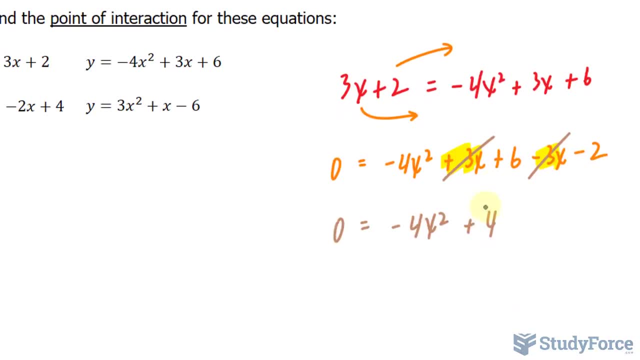 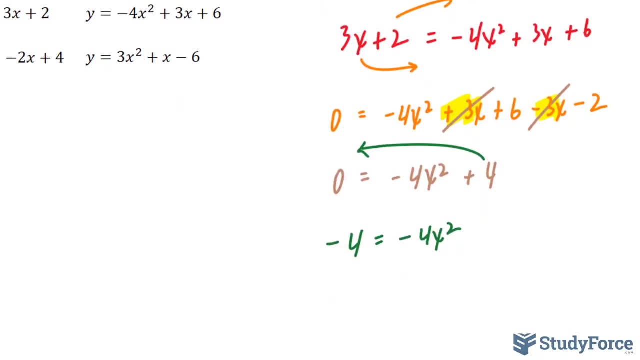 6 minus 2 makes positive 4.. Now we have negative 4x squared plus 4. We have to solve for x And for that I'll bring that positive 4 over. It becomes negative 4. That is equal to negative 4x squared. 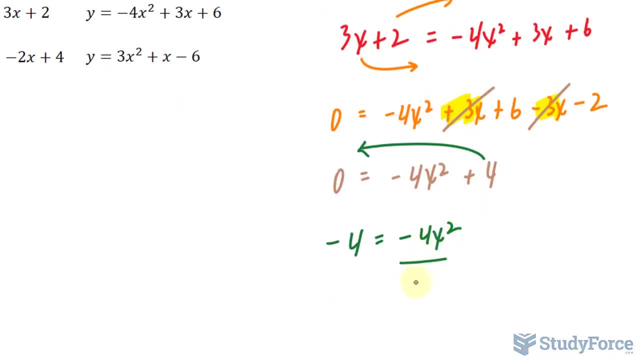 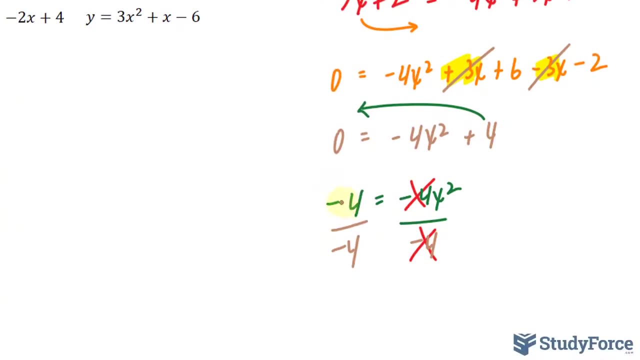 Dividing both sides by negative 4 to isolate for this x. So by dividing both sides by negative 4, this negative 4 and that negative 4 cancel out. And negative 4 divided by negative 4 makes positive 1.. So positive 1 is equal to x squared. 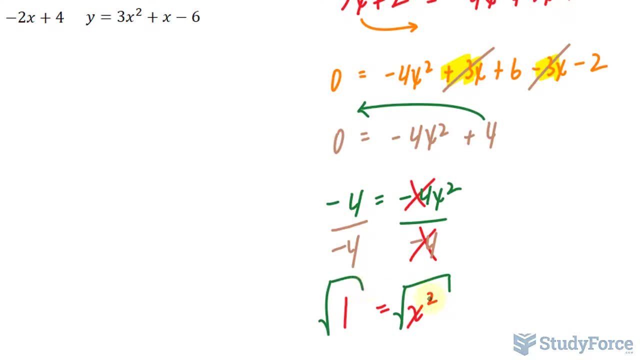 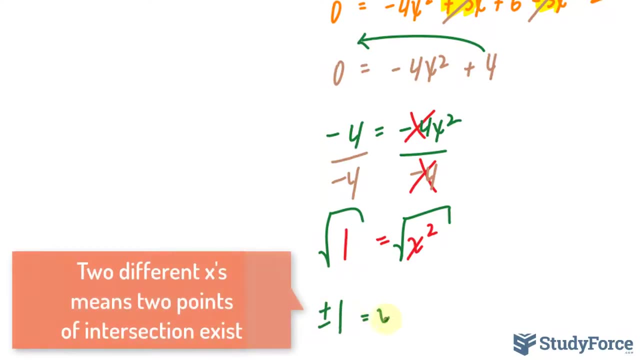 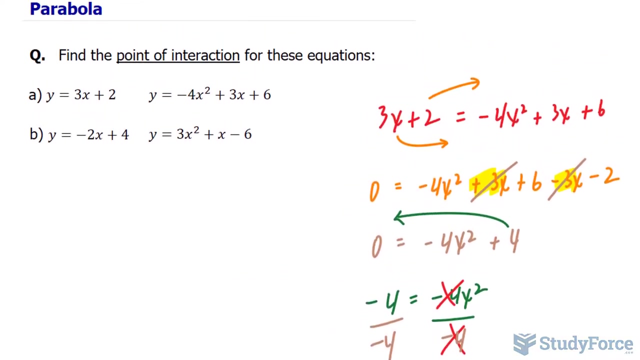 Square rooting both sides. This will eliminate this exponent of 2.. And the square root of 1 makes plus minus 1.. This means that we will have two points of intersection. I'll take plus 1 and minus 1 and substitute them into this equation. 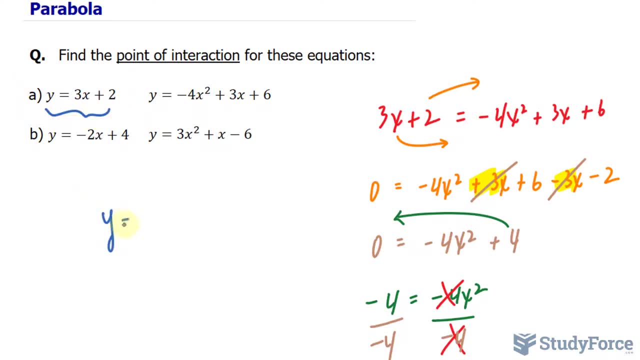 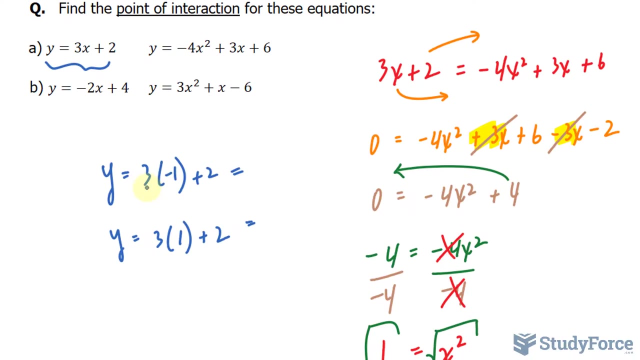 to get their corresponding y coordinates. y is equal to 3 times negative 1 plus 2.. And y is equal to 3 times positive 1 plus 2.. Let's answer both of these 3 times negative. 1 makes negative 3 plus 2.. 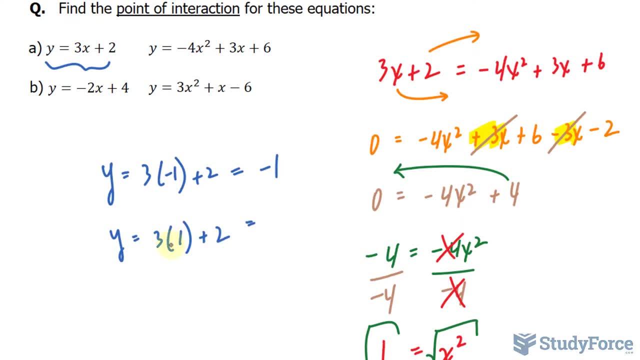 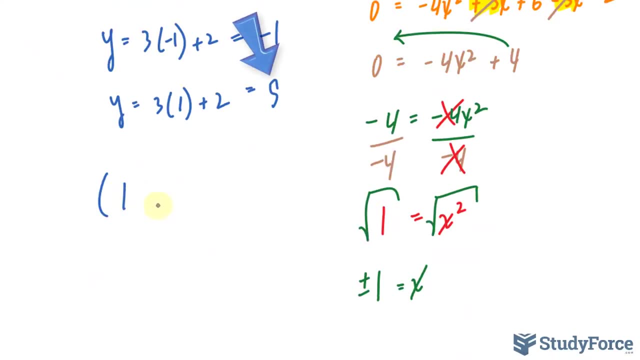 y is equal to negative 1. And 3 times 1 is 3 plus 2 is 5.. Our two points of intersection are 1 and positive 5. And the other one is negative: 1 and negative 1.. A graph of these two equations is shown on your screen.